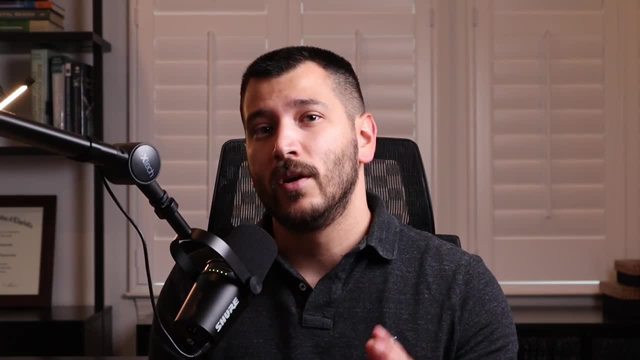 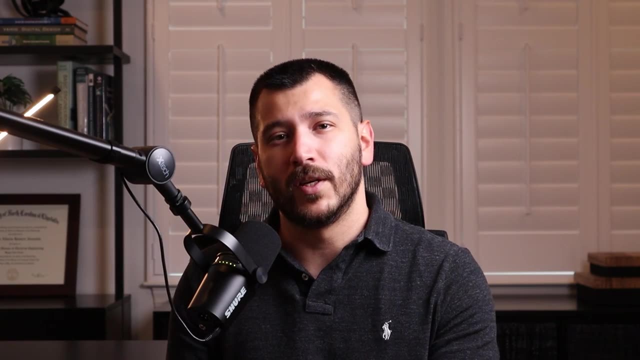 scheme. So in this video I'm going to be showing you how to set up a breaker failure scheme for the feeder breaker at a 230 to 13.8 kV substation. So in order to set up a breaker failure scheme, we need a few pieces of information. First, we need to know when the breaker has been told to trip. 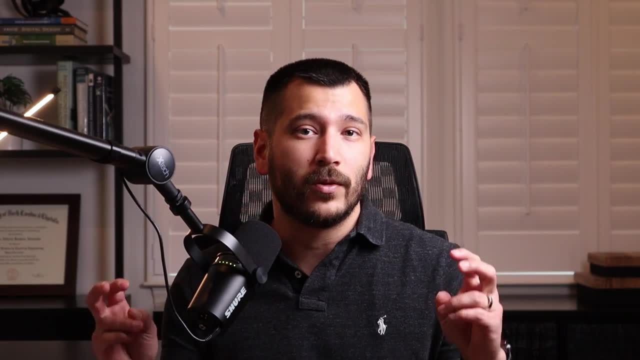 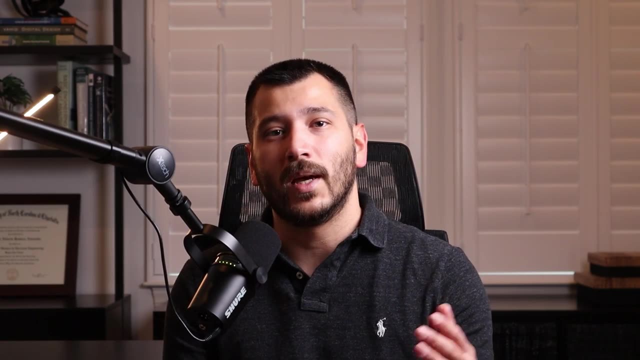 by any relay at the substation. So this is what we call the breaker failure initiate signal and it basically tells the relay that's doing the breaker failure protection when the breaker has been told to trip by any relay at the substation. Second, we need to know how long the breaker should take to trip following a fault. This is what we 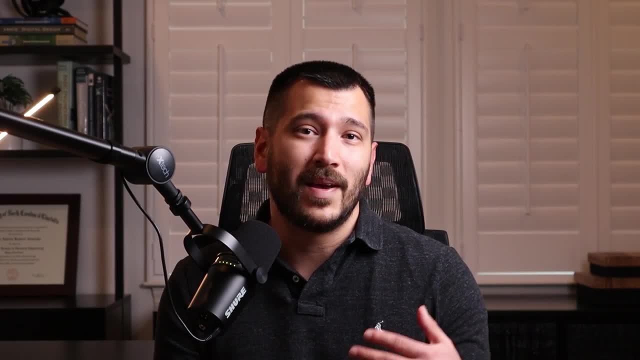 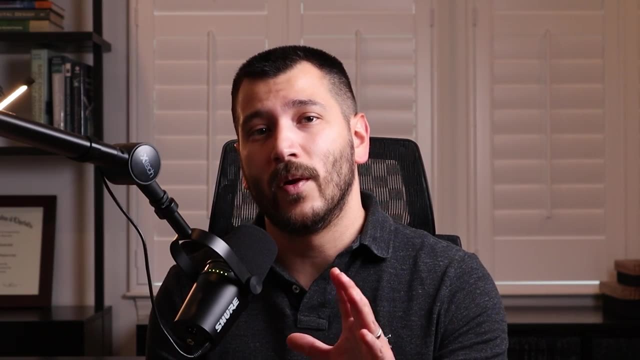 we call the breaker clearing time. this is a specification of the breaker and it basically tells us how long the breaker should take to trip once its trip call has been energized. and then, third, we need to have a way to know whether the breaker has successfully tripped or not, and we 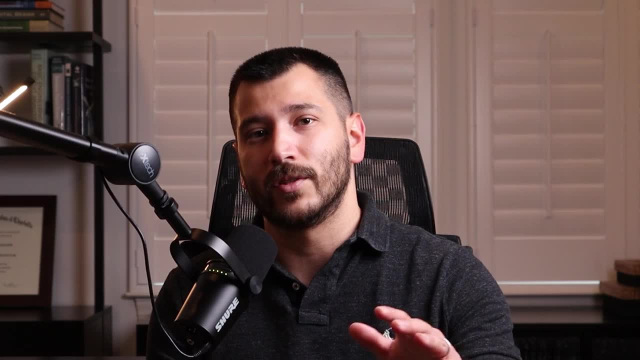 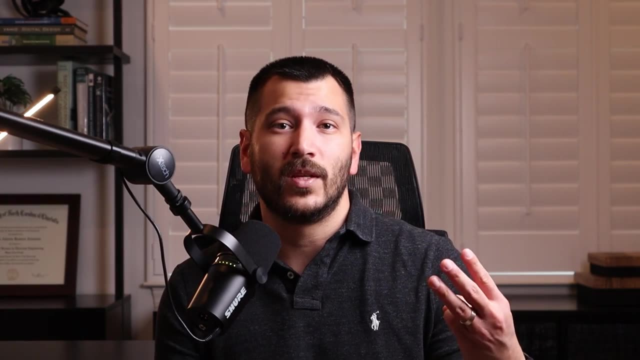 can use the breaker's 52a status for this, which basically tells us if the breaker is closed or open, or we can use the current that's flowing through the breaker, as this will tell us if it has cleared the fault. so again three things. we need to know whether the breaker has been told. 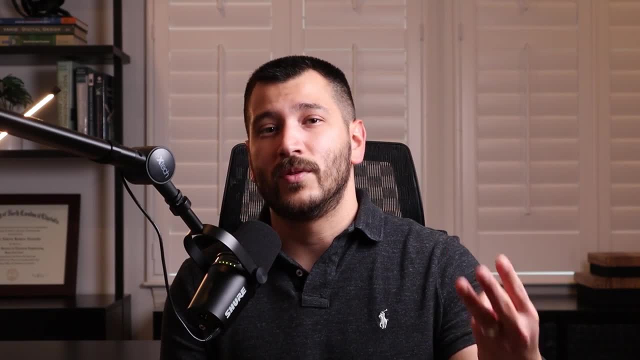 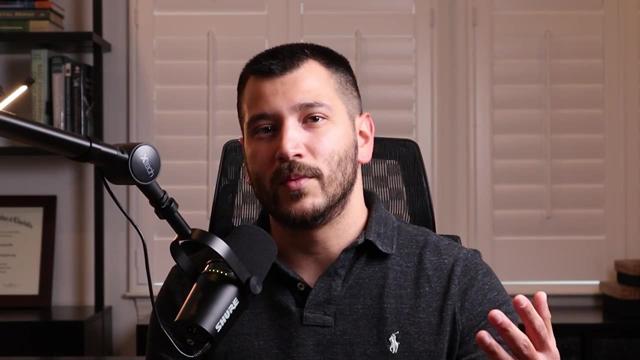 to trip. we need to know what the clearing time of the breaker is, and we need to determine whether the breaker has successfully tripped or not by looking at the current that's flowing through the breaker. now, before we go deeper into how breaker failure schemes work, make sure to download our 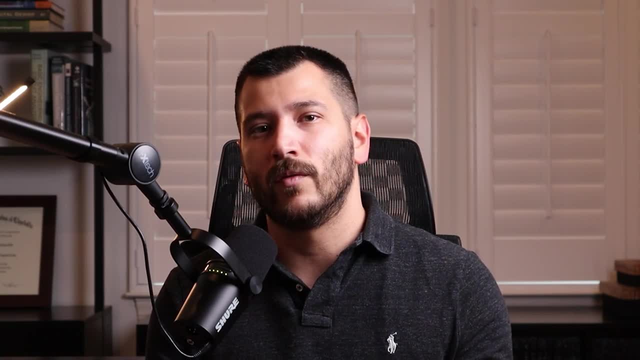 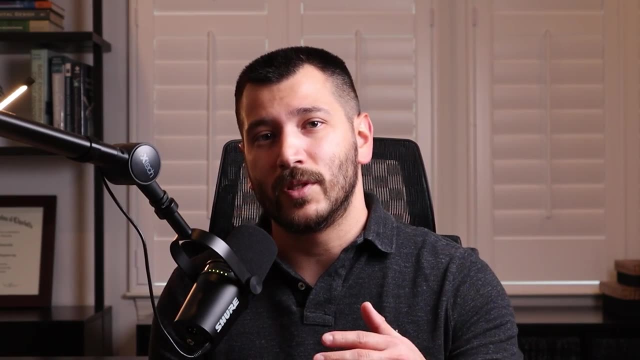 protection and control: fundamentals pdf. it's a 28 page pdf where we cover all the basics about power system protection and control. make sure to check it out. the link is in the description below. all right, so let's take a look at an example: 230 kv to 13.8 kv substation that has five feeders. 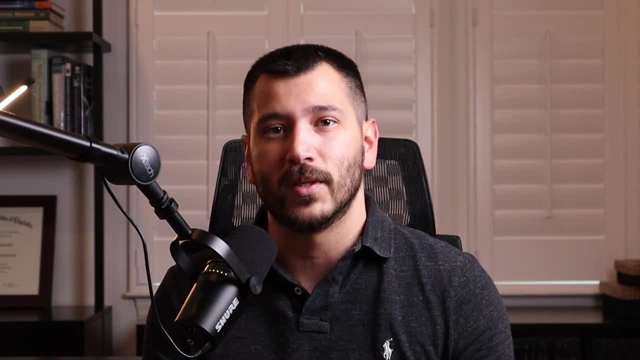 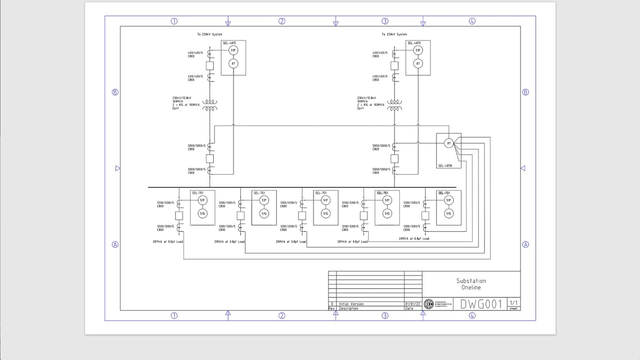 and we're going to be implementing a breaker failure scheme for one of the feeders at the substation. so, for example, let's say that we have this substation and we want to implement a breaker failure scheme using this scl751 relay on the bottom left feeder. so this one that i have over here on the screen. 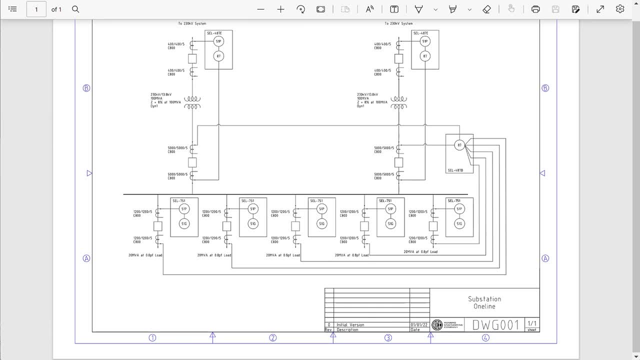 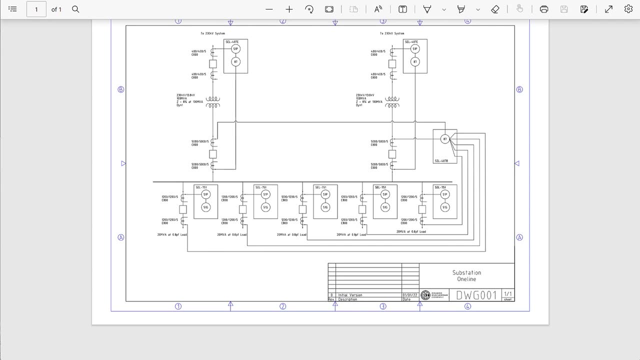 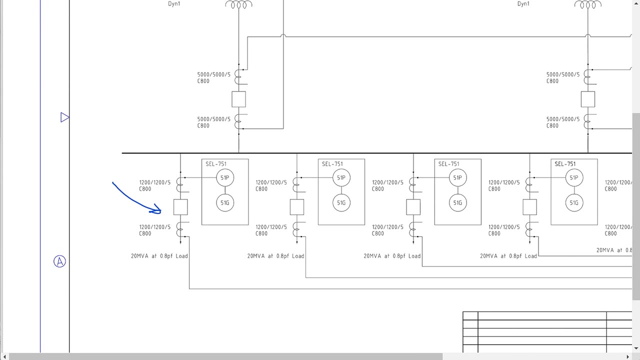 the bottom left feeder. and again, this is a 230 to 13.8 kv substation. it has two transformers, one 13.8 kv bus and then five feeders off of the substation. so we're going to be implementing the breaker failure scheme on this breaker over here. so the bottom left feeder now, in this case. 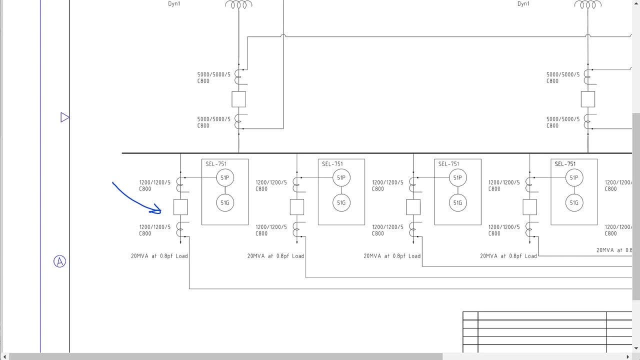 the scl751 relay is implementing protection for the distribution feeder as well. so it will tell the breaker to trip if it detects a fault in the feeder. so again this feeder goes to a distribution system and if there's a fault here in the feeder, this scl751 relay will trip this feeder breaker. now this breaker can also. 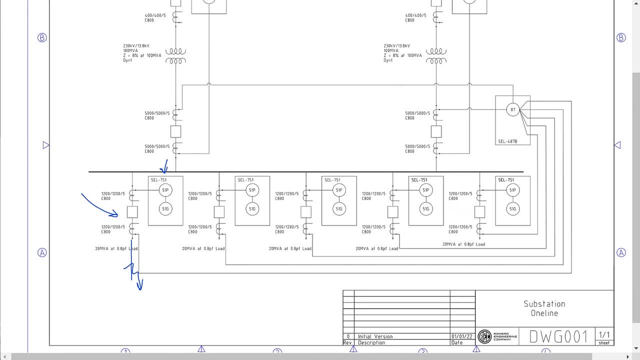 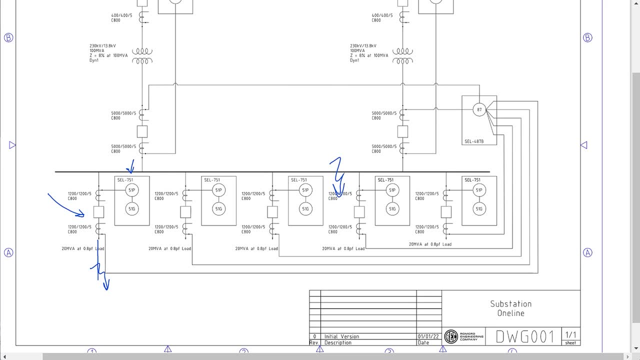 be tripped by the bus differential relay and scl487b for this substation for faults in the bus. so if there's a fault on this bus over here, the scl487b will see that bus fault in the bus substation over here, the scl487b will see that bus fault and it will trip all the breakers that are. 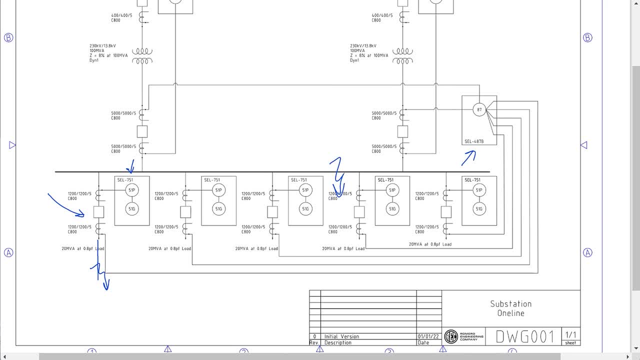 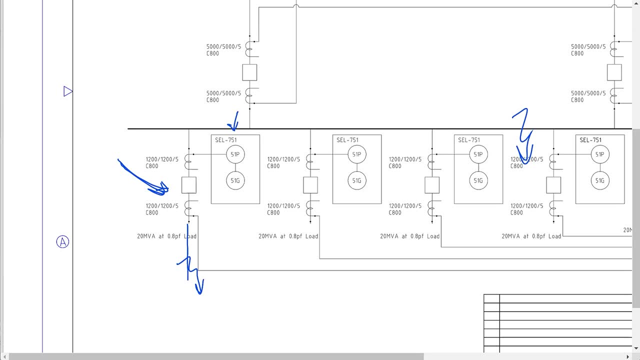 surrounding that bus. so the key point that i want to make here is that the feeder breaker that we're implementing, the breaker failure protection for again this one over here- can be tripped by both the scl751 feeder relay and the scl487b bus relay now in order to implement. 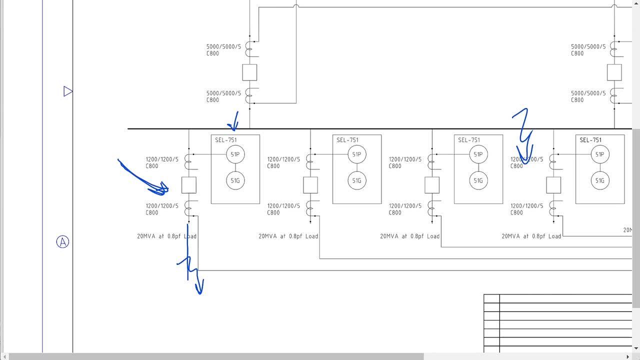 the breaker failure scheme. we need to know when the breaker has been told to trip, no matter where the trip came from. so in this example, then, we will have two bfis, and a bfi is what we call our breaker failure initiate signal, and we're going to have two of them again, one from the 751 and 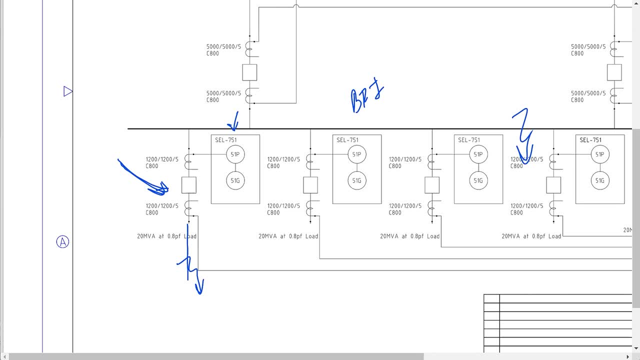 one from the 487b. now, for this example, we're going to assume that the output from the scl487b that is being sent to the scl751 for a breaker failure initiate signal is going to be input 101. so when input 101 on the 751 relay is a logical one, that means that the scl487b 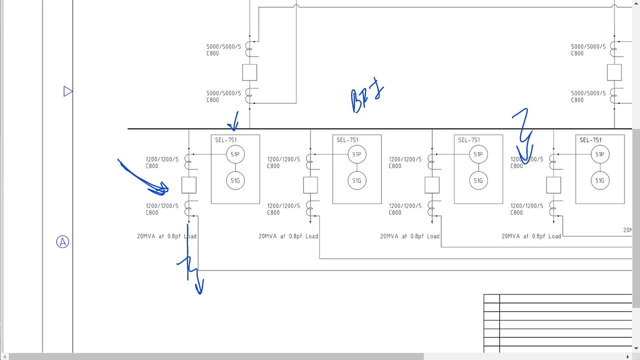 relay has told the feeder breaker to trip. now the other thing that we need to know is how long to wait before we check to see if the breaker has successfully tripped following a fault, and this is what i talked about a few moments ago, which is what we call the clearing time of the feeder. 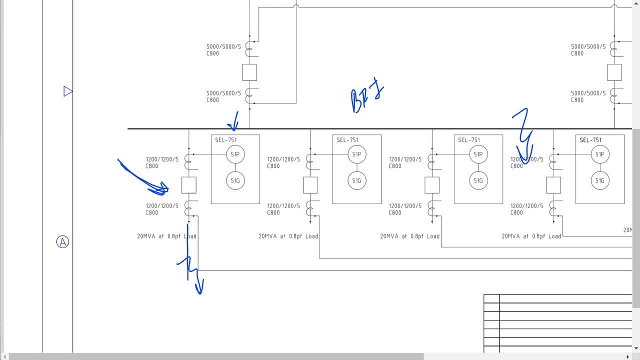 breaker, meaning the time that it will take for it to open once its trip coil has been energized. now, typical clearing time for a distribution feeder breaker is somewhere around five cycles. transmission breakers can have typically a faster clearing time, usually around two to three cycles. five cycles is somewhat normal for a distribution feeder breaker. 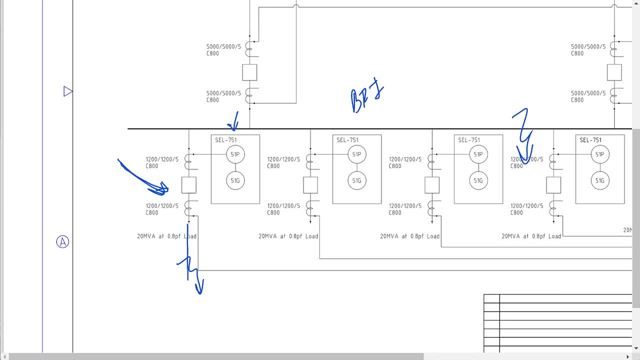 now, this information is specific to each breaker, so you need to look at the nameplate for each breaker to see what the current time for that specific breaker is. so in this case, if we expect the breaker to clear within five cycles, we can set our breaker failure timer at around 10 to 12. 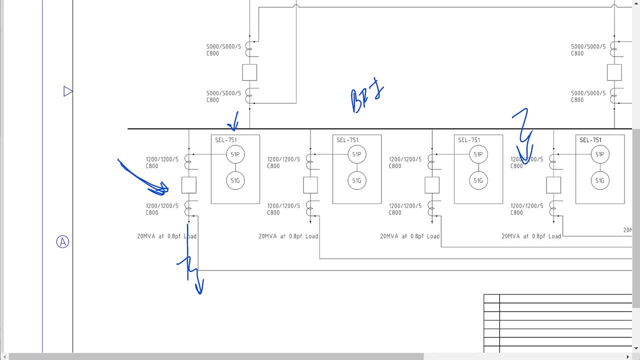 cycles. this will allow enough time for the trip signal to get to the breaker strip, coil the breaker to open currents to subside, plus some margin, of course, above this number. so in this case we're going to use 12 cycles as our breaker failure time again. this is how long. we're going to take to declare a breaker failure. now the breaker should technically take around five cycles to open once it's been told to trip. now, in this case, the scl751 relay would have to trip all the surrounding breakers, in this case the other four feeder breakers and the two main. 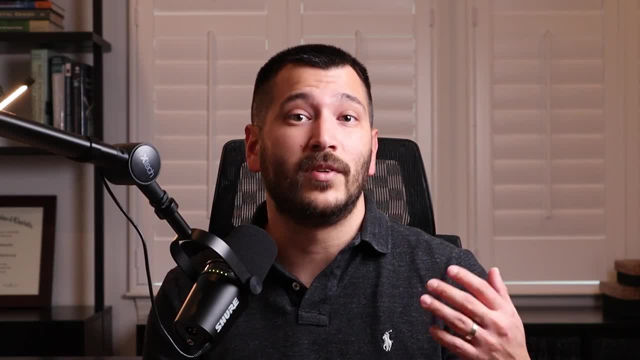 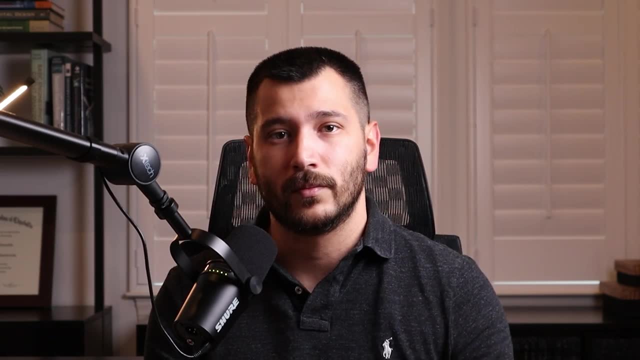 breakers on the low side of the transformers. now, for this example, we're assuming that the feeder is going to have to trip anything downstream of that feeder, because there's no source downstream of the feeder that can feed the fault. now there's many ways that we can implement this tripping of the 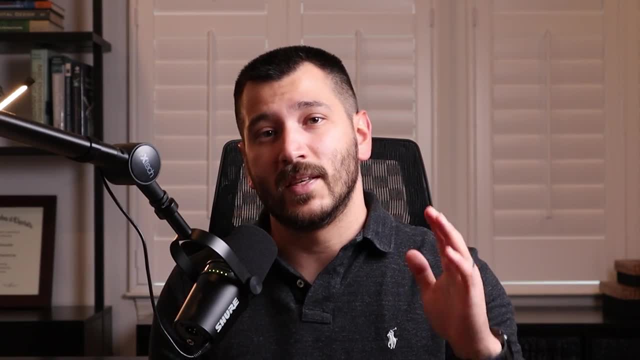 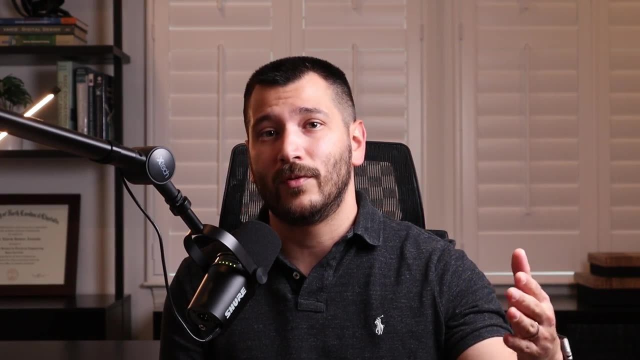 surrounding breakers. one option is just to take several outputs from the scl751 relay and trip individually each one of the breakers. now this option is often not practical because we would have to have one output from the relay to trip each one of the breakers. now another option is: just to take one output from the relay and trip a lockout relay that will then go ahead and trip each one of the breakers individually. so essentially, we're using a lockout relay as a contact multiplier from our breaker failure relay. all right, so that's the theory about breaker. 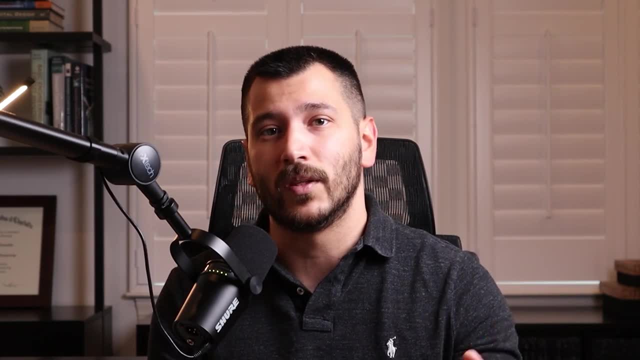 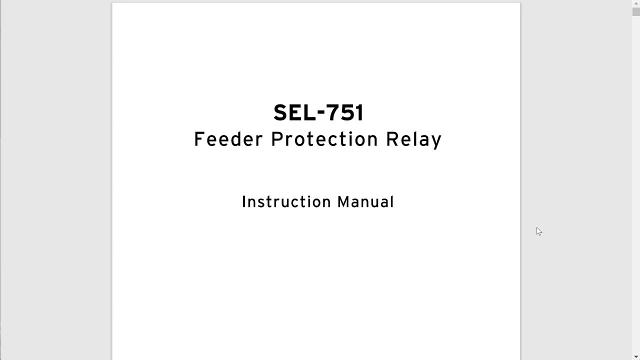 failure protection. now let's see how we can implement this in the scl751 relay. so before we go into the programming of the relay, let's first take a look at the instruction manual for this scl751 relay. i always say this, but it's very important that you always take a look at the 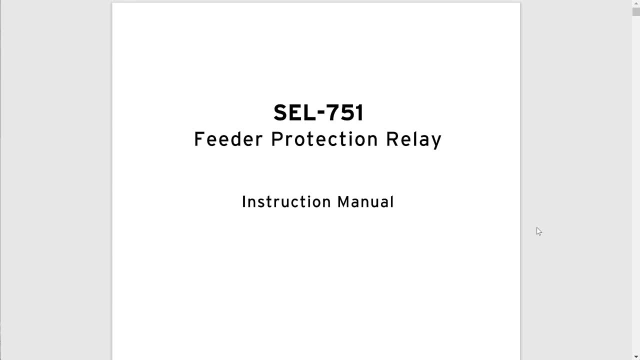 instruction manual for the relay that you are using, and this is because different relays, even from the same manufacturer, can implement schemes differently. so if you have a 751 relay, that might be different than, say, an scl451 relay, for example. now what i have here is the instruction manual for 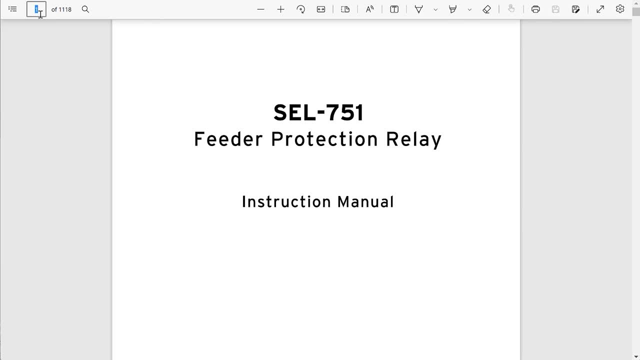 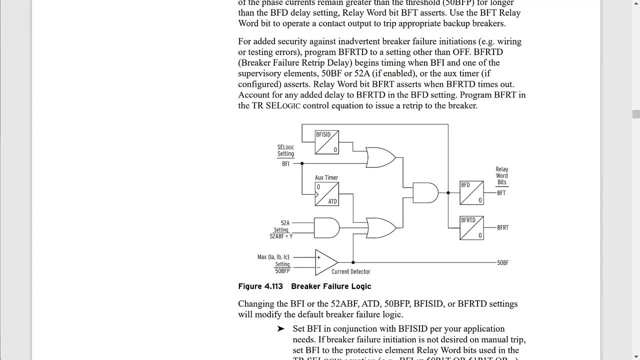 the scl751 relay and if we go to page 341 we can see the breaker failure logic over here. so let's go through how this scheme works so that we know how to program the relay. now we can see here that we have the bfi signal over here and again this is what tells the relay when the breaker that we 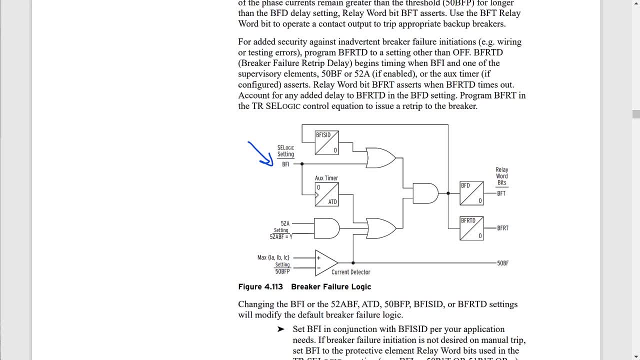 are doing breaker failure on has been told to trip. in our case, we said that this scheme can be used to come from two relays, the scl751 for the feeder and the scl487b for the bus. so we're going to trip this breaker both for feeder faults and for bus faults. so, for example, in our case we can then 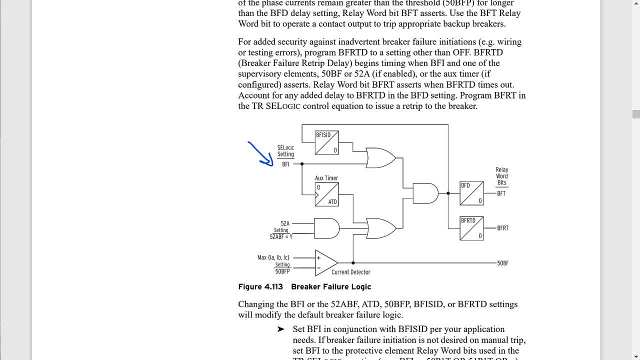 program, our bfi equation, the breaker failure initiate equation to something like our trig, and this is basically rising trigger of trip, which is going to be the internal trip from the feeder relay. or, same thing, rising trigger, input 101, which we said was the input from the scl487b relay, that tells the scl751 relay that the 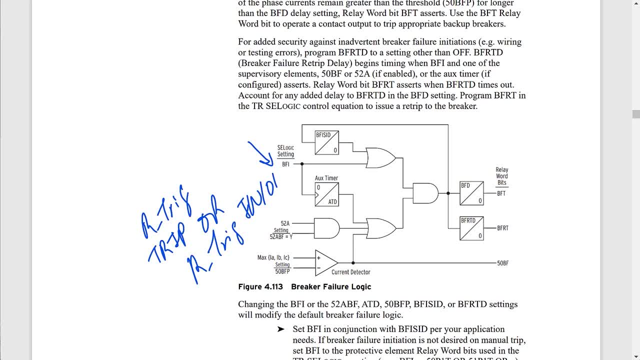 scl487b relay told the breaker to trip. so when the scl487b declares a trip, it's both going to trip the breaker directly and it's going to send a signal, which is input 101 on the scl751 relay to tell it that it told the breaker to trip. so this is our bfi that's coming from the scl487b relay. now let 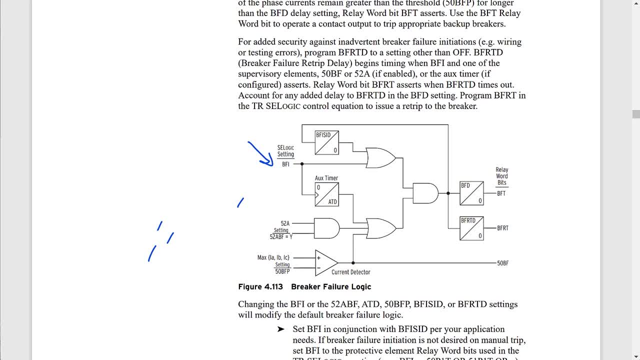 me get rid of some of these over here so we can talk about the rest of this logic here. so let's go back to the logic scheme. you can see on this part over here that the bfi signal will seal in if there is current, if we are using timer atd or if we are using the 52a interlock function, 52abf. so that's. 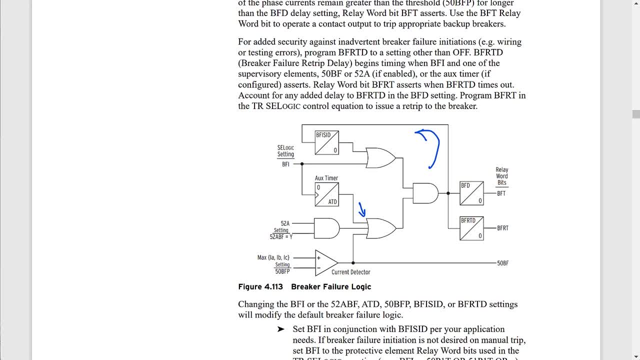 these three conditions that i have on this, or gate over here. so, essentially, if we have a bfi signal that's going to come to this end gate over here, and if this part of the end gate is true, then the output of that becomes a logical one and it's going to seal in this way. so, basically, once we receive, 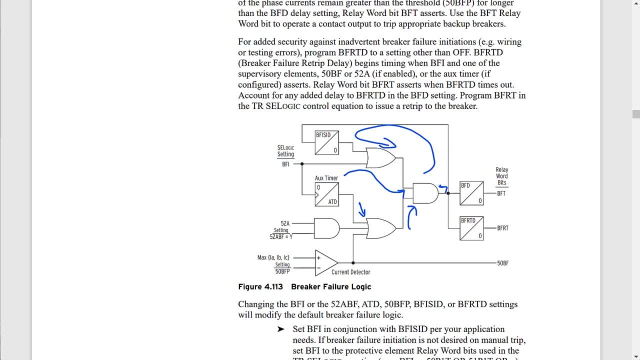 a signal. that signal is going to be maintained until we break it, with one of these three conditions. so let me get rid again of these arrows over here. and, for simplicity, for this example, we're going to set the timer atd to off, so essentially we're getting rid of this portion. 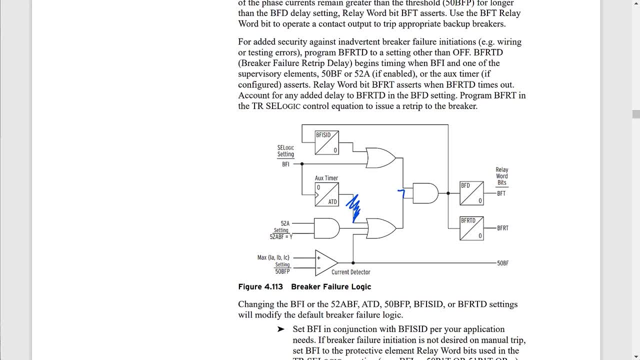 of the logic and we're going to set the 52abf setting to no so that we get rid of this portion of the logic as well. and i'm doing this so we can focus on the typical breaker failure scheme where we're seeing those two kind of conditions. okay, so we're going to put in the storm pattern. 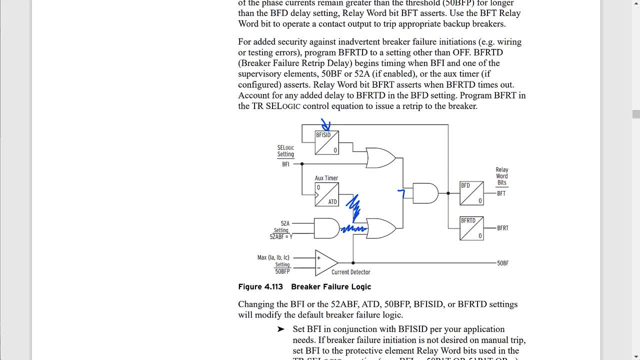 here and we're going to call that bfi signal and then we're going to create this new yourself and in this case we're going to use the time frame over here that we gave for호 duck. so if we conetto f is being an postal on five time frame, number five, we can say that this is other world. 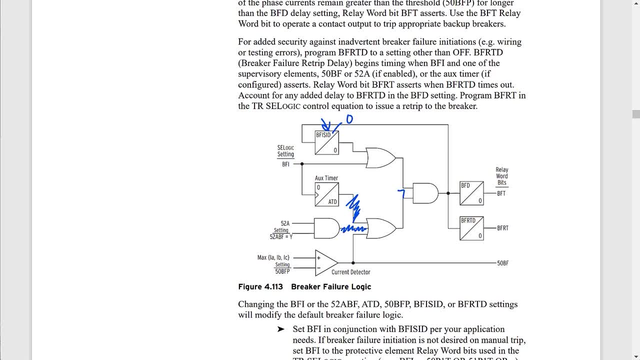 so we'll pride this parameter. it's going to be a portion of service height and this condition is not going to have a time frame of six, and this will be Them what's going to want me to say okay with that. okay, let's try it again. 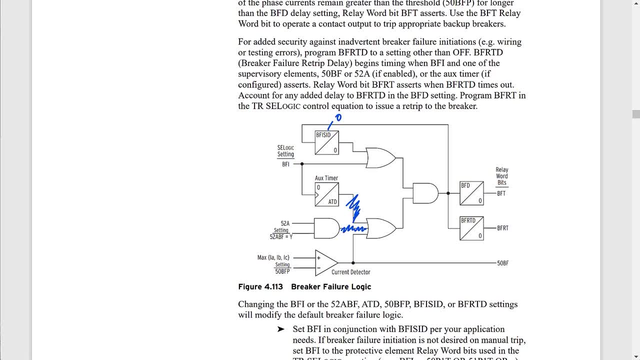 we're going to assume that we're going to set this to zero, and let's say that the pfi signal becomes a logical one. provided that there's current flowing through the breaker, the output of this n-gate is going to become a logical one over here, which means, then, that this input to this or gate 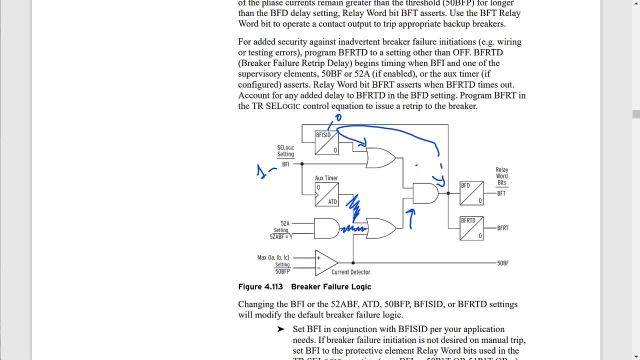 over here is going to be a logical one now. so this is a way to essentially seal in the bfi signal, meaning once we get it we're going to continue to assert this part of the n-gate continuously, even if the bfi signal now goes to a logical zero. so even if the bfi, the asserts now we also have 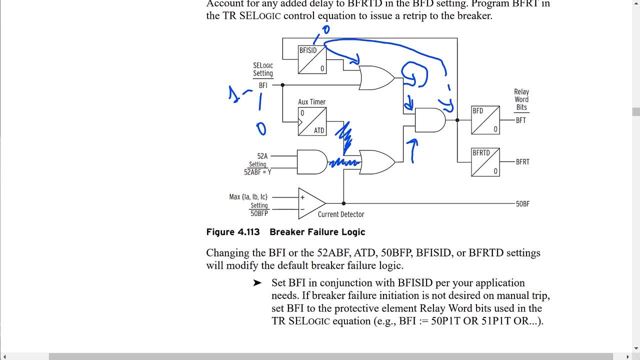 setting 50 bfp down over here. and this is the breaker failure current detector. this is what we use to determine whether or not the breaker has successfully cleared the fault. in other words, if we see current flowing through the breaker, then we know that it has not opened. now there are 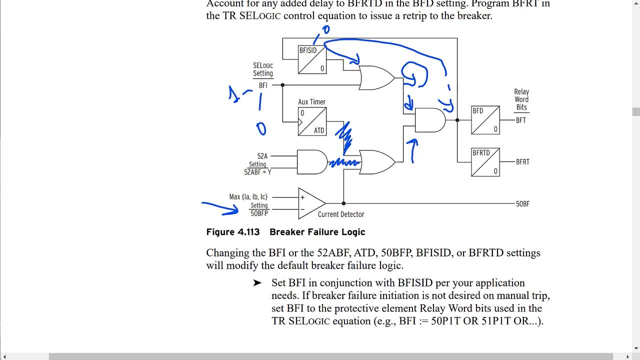 different philosophies for setting this threshold. some engineers like to set it above load but, of course, below fault current levels, while other engineers like to set this as sensitive as possible. this is basically the comparison with measured currents that tells us if there's current flowing through the breaker. 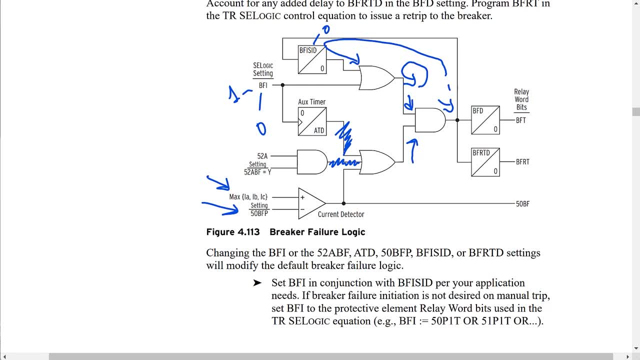 now there are pros and cons to setting this very sensitive or setting it less sensitive above load. so, for example, if you set this threshold above load, you run the risk of having a restricted fault that may have a very low current level and you may not declare a breaker failure. 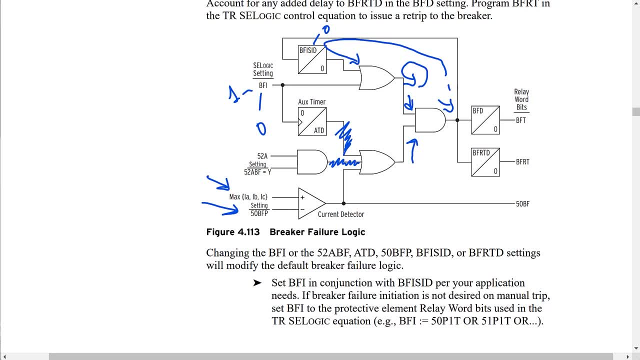 on that condition, even if the breaker fails to open following a trip. however, the pro of this is that this portion of the logic, the bottom portion of this and gate over here, will not be picked up always, which may be an issue if you get a wrong bfi signal. 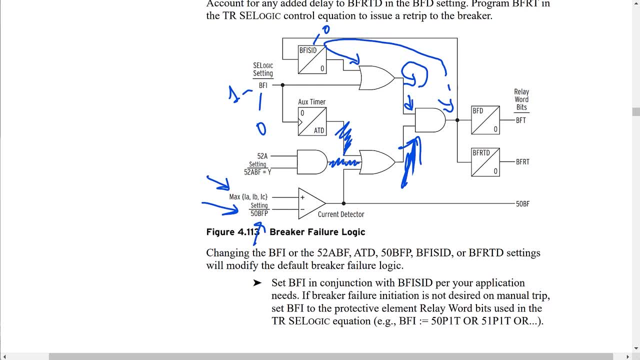 so, in other words, if you said this too sensitive, that might mean that any little current under normal conditions will cause this comparator to be a one, which means that this input to the orchid is a one, which means that this part of the logic, the bottom input to this angle, is always going to be a logical one, and so if you get a wrong one over here, 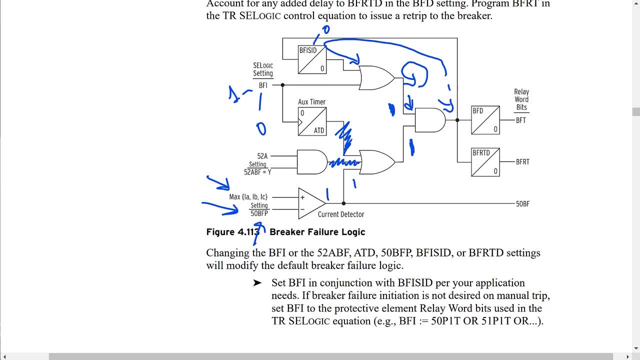 signal you may trigger a breaker failure condition by mistake. now the pro of setting the 50 bfb- setting very sensitive- is that you don't run the risk of not detecting a fault. but again you do run the risk of declaring a breaker failure if the bfi is received by mistake. now i'll say this. but 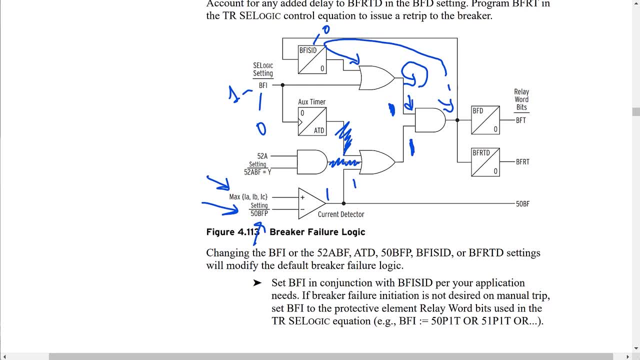 we're going to talk about the re-trip function here in a second, which alleviates this concern. now, the point that i want to make over here is that there is no right or wrong answer here. it really depends on your specific application and risk tolerance. personally, i prefer to set. 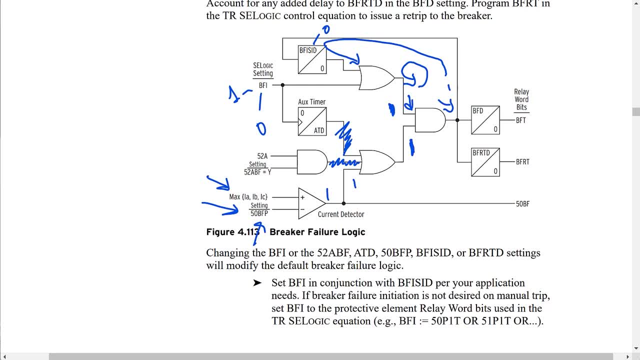 the 50 bfb threshold low, provided that we use the re-trip function, which errs on the side of dependability rather than security. now, for this example, we're going to set this threshold at the minimum possible setting, which is 0.1 amps secondary. so this setting is going to be 0.1. 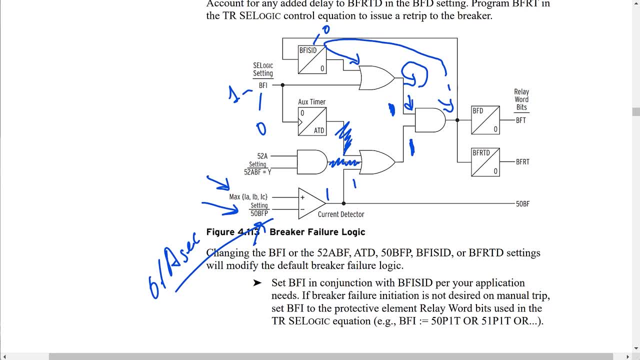 amps secondary. and again, let me get rid of all this over here and again, i mentioned the re-trip function, but now let's talk about it in a little bit more detail. so this timer over here, bfr td, is the breaker failure, re-trip delay. this is an important function that we should always 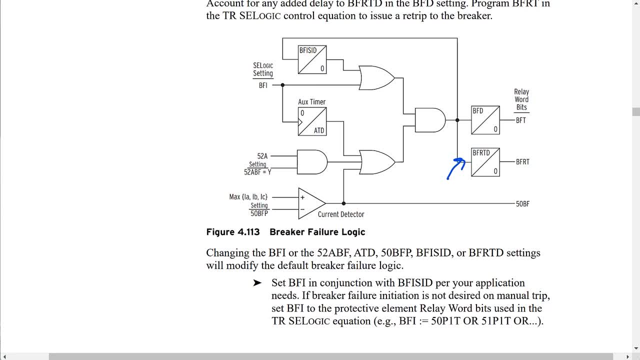 use. in my opinion, what this is is, if we get a bf initiation, if we get a breaker failure initiation, in other words, if we are now timing on the breaker failure scheme, we will go ahead and try to re-trip the breaker immediately or at least with a very short time delay, since, after all, if we received 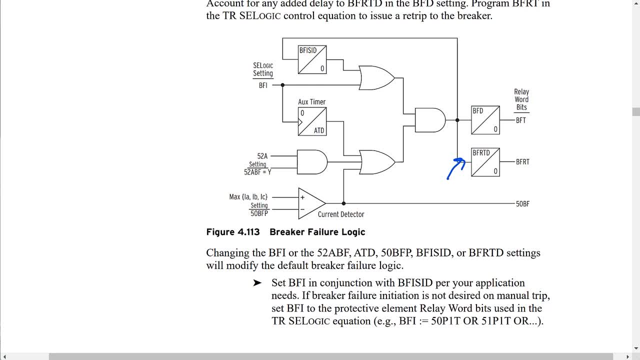 the bfi signal, the breaker must have been told to trip. that's the whole premise of the breaker failure initiation. and this is done to potentially avoid declaring a breaker failure trip for a false or erroneous bfi signal. so, for example, let's say there's a problem in the wiring that's coming from the 47b. 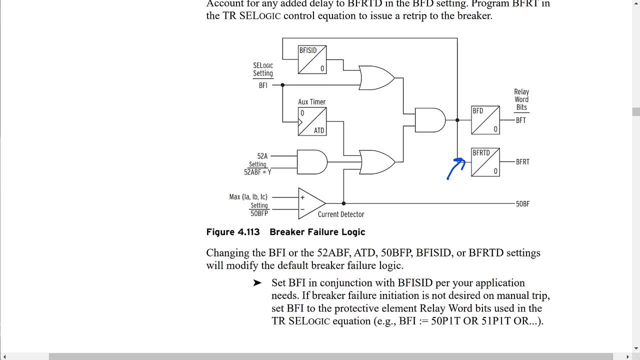 relay to the 751 relay and the relay thinks that the input in 101, in this case, is energized and, again, assuming that this is a problem with the wiring, not actually a trip signal from the 47b. if this is the case, then the scl. 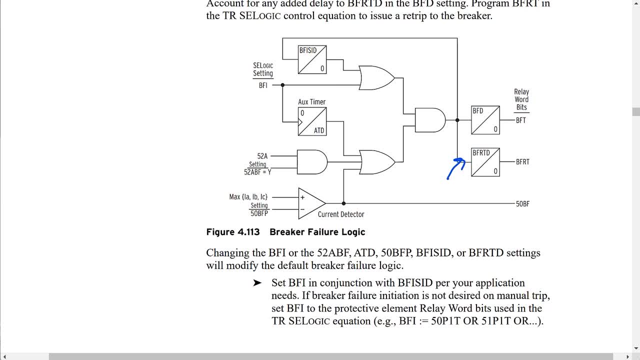 51 will start timing on the breaker failure scheme because it's going to get the bfi signal, it's going to see current. that's a logical one, logical one, output of this angle is a logical one and it's going to start timing on the breaker failure signal and it will eventually time out. 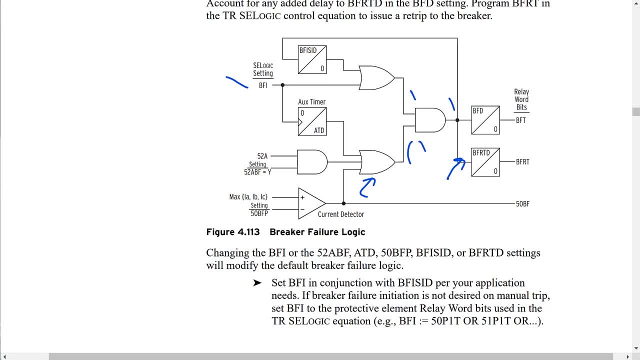 because it's going to see current flowing. because, again, the reason why we got the bfi from the 47b was because of problems in the wiring, not because the 47b actually told the breaker to trip. so this is just a case where the re-trip function is helpful. 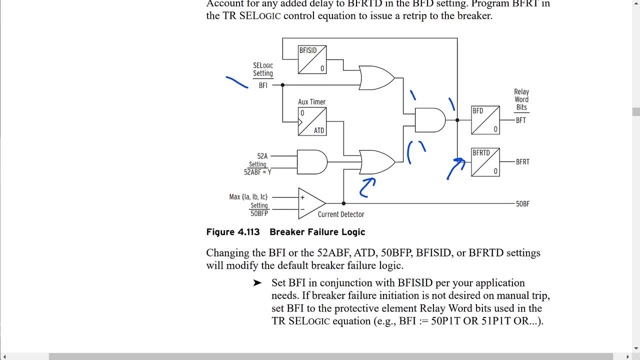 because now we can go ahead and say: well, if you initiated breaker failure, go ahead and try to trip the breaker again, because again, after all, if you got the bfi signal, it's because the breaker was supposedly told to trip already. so go ahead and try to re-trip the. 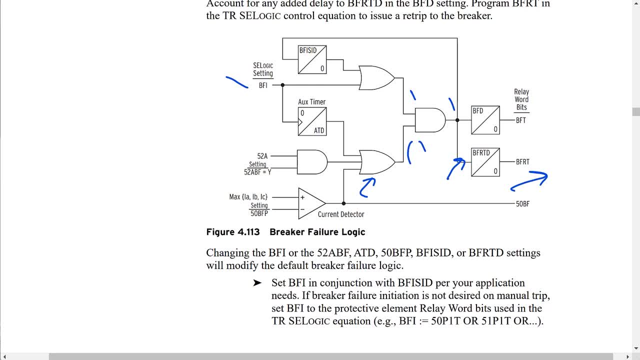 breaker and if you did get the bfi signal by mistake, the worst that's going to happen is going to trip this one breaker. of course that's not ideal, but it's better than declaring a breaker failure. that would potentially trip the entire bus at the substation. so this is an important 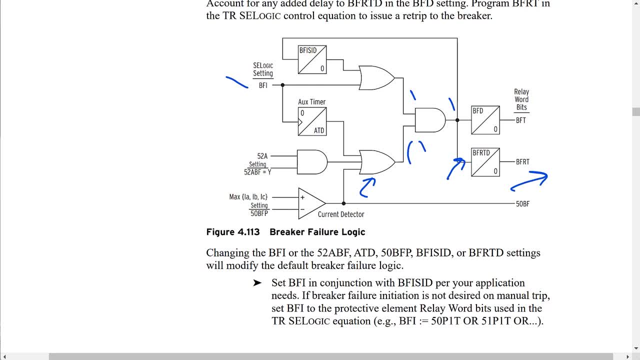 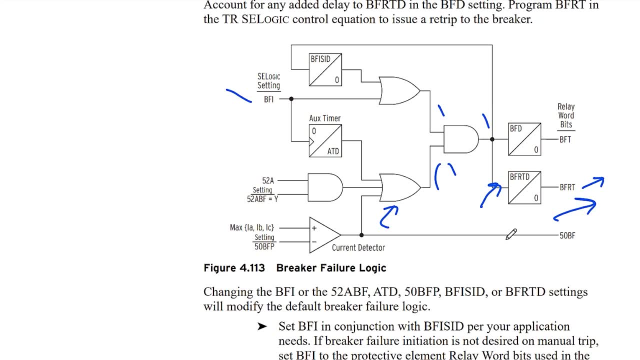 function. i always like to use it and basically what we would do is we would program it and we would call callchef to trigger this particular output here and recall this output out. we would involve bf- rt, which stands for breaker failure, re-trip- to an output that trips only. 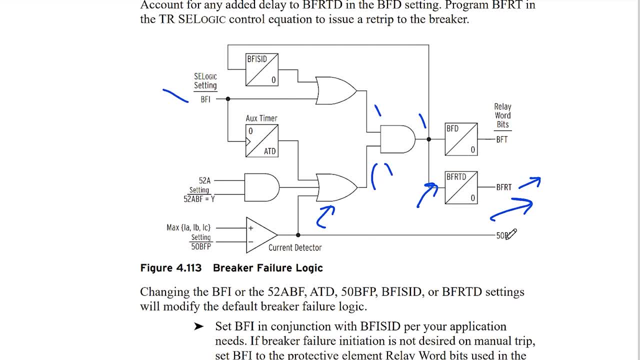 this breaker. now for our example, we're going to assume that this is output out 102, and again, this is a trip signal directly to this one breaker, not to the breaker, failure lockout. and then, lastly, of course, we have the breaker failure time delay, pfd, and remember that. 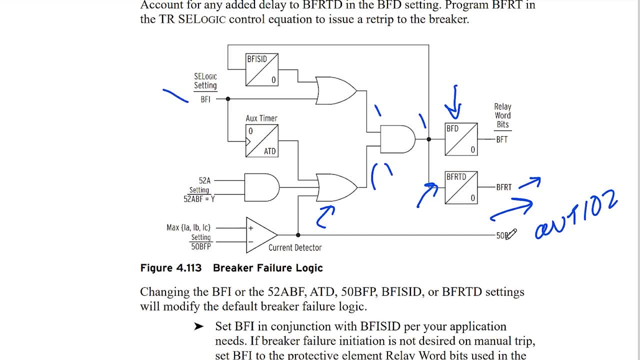 this is the time that we will wait to declare a breaker failure, trip following a trip. if we still see current flow and we want to go ahead and actually display this output, that just is the time that we will wait to declare a breaker failure, trip following a trip, if we still see. 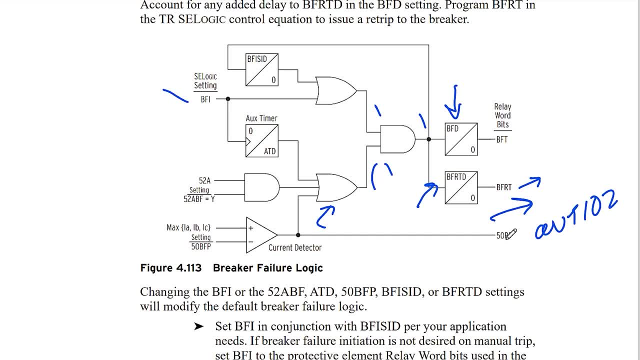 current flow and we feel the error of the calGM. we're saying, instead of lamp shooting through the breaker. so in our example we will set this to 12 cycles, which is 0.2 seconds, and again, this is assuming that our breaker has a clearing time of five. 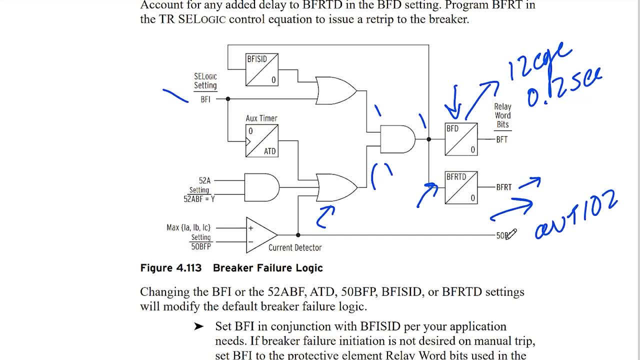 cycles, meaning if the breaker works as it's supposed to, it should clear the fault in five cycles. so we're gonna wait until 12 cycles just to give some margin, before we declare a breaker failure and trip all the adjacent breakers. now the output of this logic is this really work? but over here, BFT we can also make use. 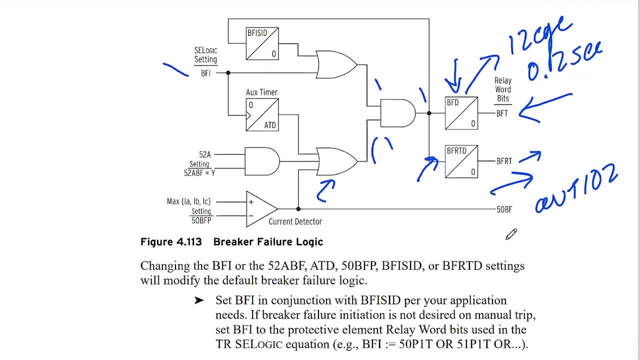 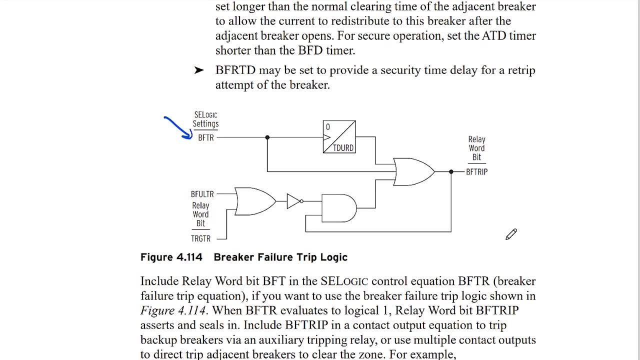 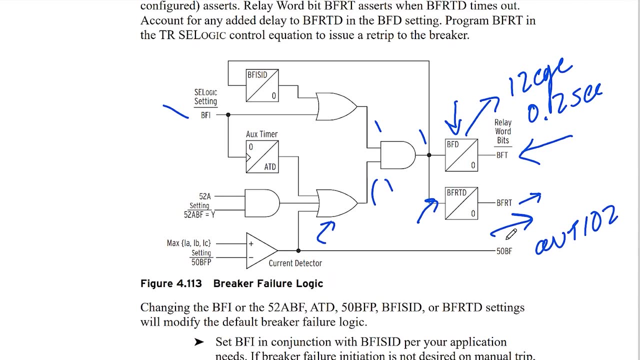 of a built-in breaker for your trip logic which is down here in the instruction manual, and what we can do is we can say: well, we're gonna program this over here to BFT. and again, BFT was the output of the breaker failure logic that we had over here. and essentially we're gonna say: when we declare a breaker, 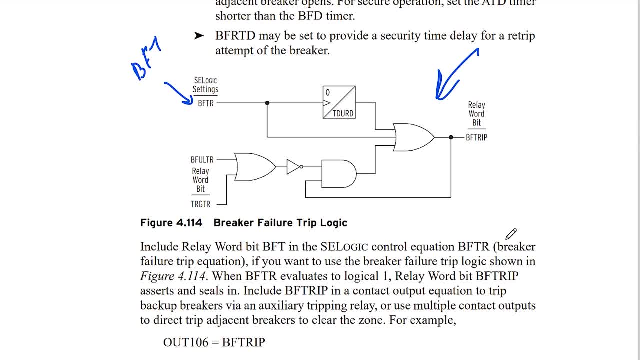 for your trip. use this built-in logic for the breaker failure scheme. essentially, all this does is it seals in the trip signal from the breaker failure scheme until you reset it manually. so it's going to continue to assert this relay orbit until you manually go and reset the relay targets. this could be done, for example: 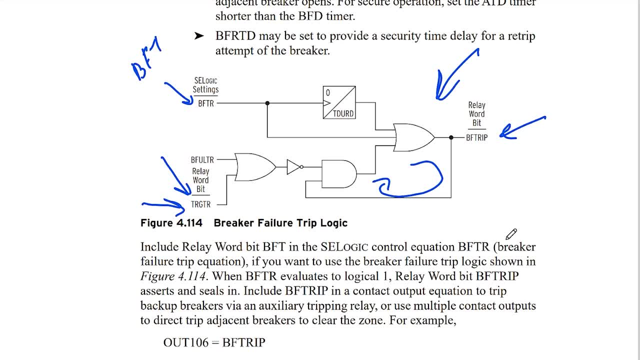 at the front panel of the relay. you can go and hit a button in the relay that resets targets. essentially is a way to reset everything back to normal. all right, so now let's program this into our settings file. now what i have over here is the default settings for an sel751 relay. 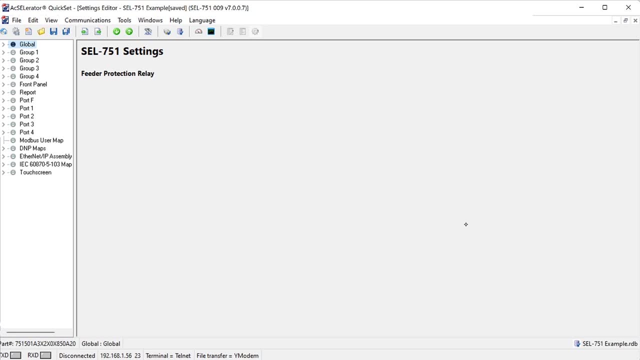 now just a note real quick before we get started here. i'm going to focus on the breaker failure settings. now, of course, if you were doing settings for a real life application, you would have to set other settings, such as the ct ratio, for example, the trip equation, the protection elements. 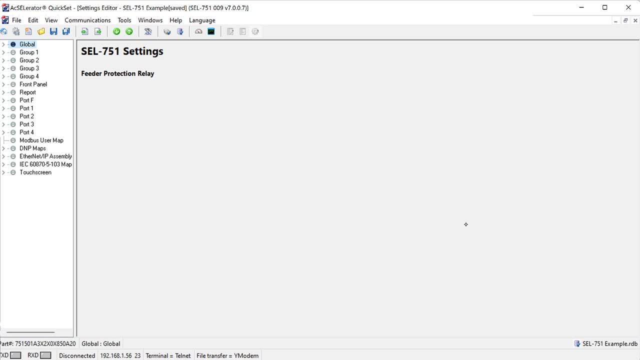 all the other settings in the relay. for this example, though, since we're talking about breaker failure, i'm going to focus only on the breaker failure settings. all right, so again, this is our default settings for the breaker failure settings, and i'm going to focus on the breaker failure. 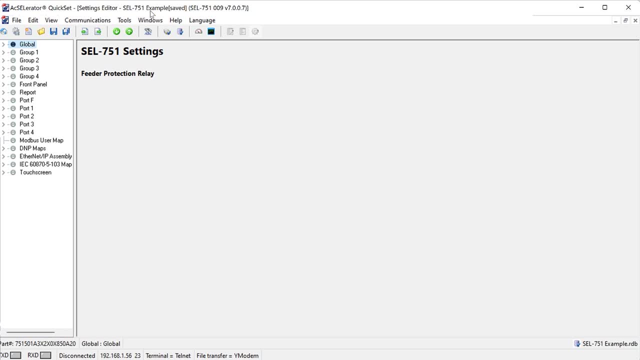 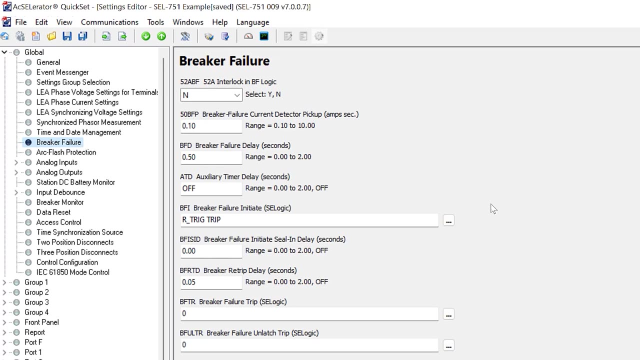 settings. and if you go over here to global- and then let me expand this- you go over here to breaker failure. this is where you configure the breaker failure scheme. again, we talked about the 52a interlock. we said that we're not going to use that in this application. that's basically a way of 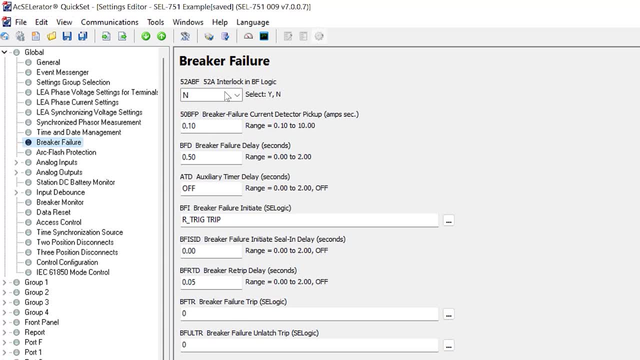 using the 52a contact from the breaker in the breaker failure logic for this example, we're just going to be looking at the current that's flowing through the breaker. we also said that for the breaker failure scheme we're going to set that at the minimum level possible. in this case it 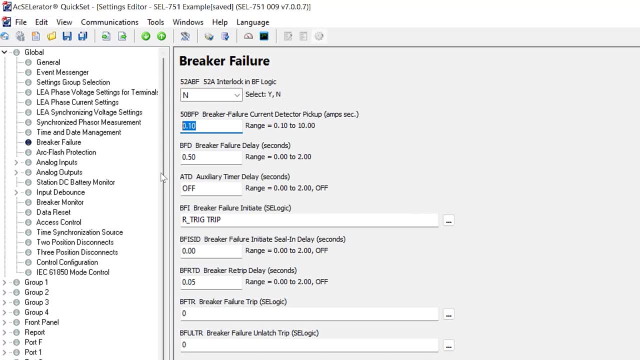 is 0.1 amps secondary. our time delay for the breaker failure scheme is going to be 12 cycles, which equates to 0.2 seconds on a 60 hertz system. of course, now we set this timer, the auxiliary timer. we're not going to use that for this example. and here is the other important setting: the bfi, the 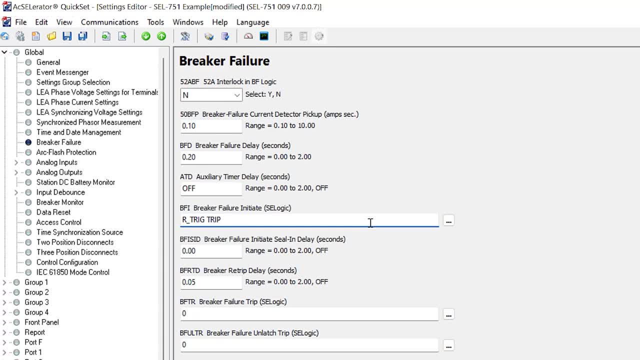 breaker: failure initiate signal. we're going to have two conditions: rise and trigger. all that goes from a logical zero to a logical one. rising trigger of the trip bit, that's essentially trips from this same relay for protective functions. or rising trigger of input 101. again, we said that. 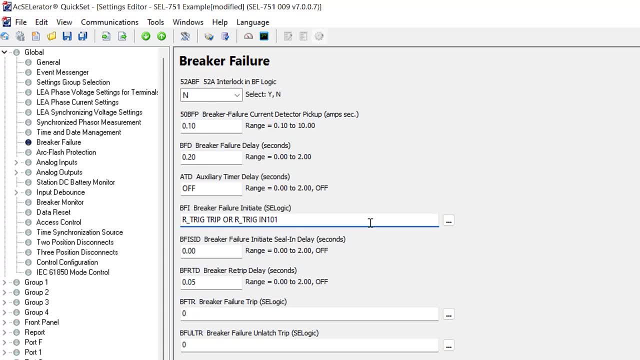 input 101 is an output from the 47b relay. that's telling the 751 relay, when it has tripped for a bus fault, the breaker failure ceiling delay. i'm going to set that to zero. basically, i want the breaker failure initiate signal to seal in right away, so i'm going to set that to zero and then. 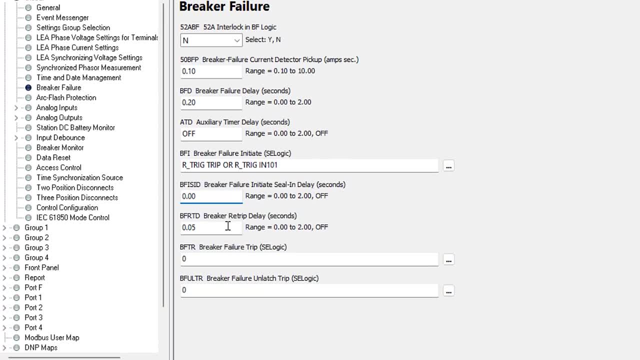 once we get it. and then we also talked about the breaker re-trip delay. this is essentially the delay by which, once we get the bfi signal, when we go ahead and try to re-trip the same breaker- i'm going to leave that at default- 0.5 seconds. that's roughly three cycles. so very, very fast and then 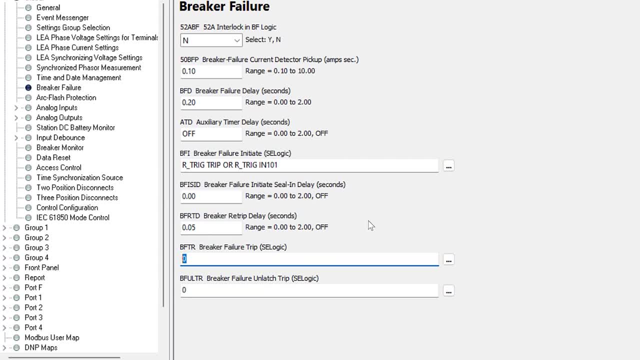 we said here that we're going to be using this equation over here, bftr, which is the built-in trip logic in the scl751 relay for the breaker failure scheme. we can program that to bft again and then we're going to use this equation over here and then we're going to use the nc relation. 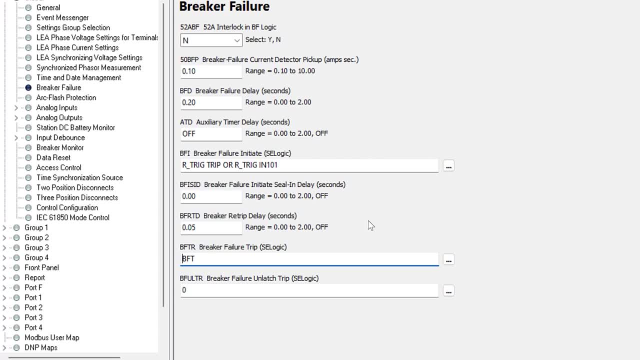 which is the output of the breaker failure scheme, which is relay warbed bft, and then it seals it in continuously until you go and manually reset the breaker failure condition. that's just a way to say: once you have declared a breaker for your trip, go ahead and seal in, because somebody needs to go and 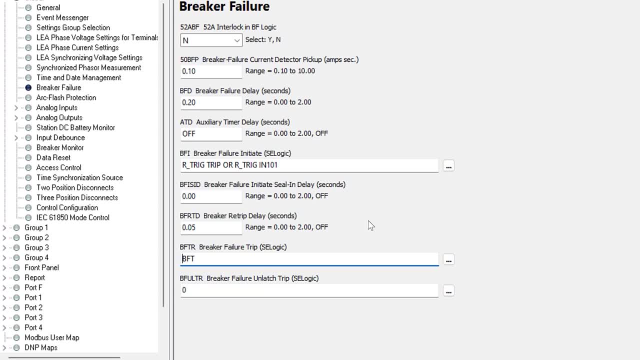 investigate what happened. and once everything has been investigated and everything's back to normal, you can go ahead and press a button on the front panel of the relay that resets this condition. and then, lastly, we have the all notch trip equation, this one over here at a zero. that's basically saying the only way to reset the breaker failure trip is to 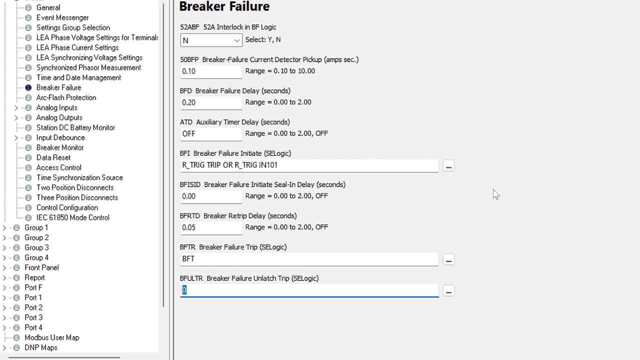 manually go and hit the reset button on the relay. Alright, so now we have set up our breaker failure scheme. the last step is to program the outputs from this scheme into the contact outputs that are actually going to go and take the actions needed. 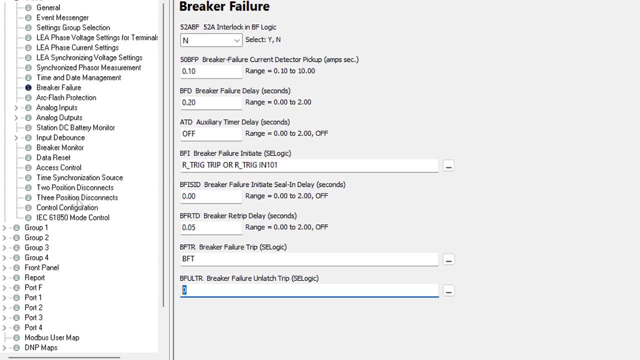 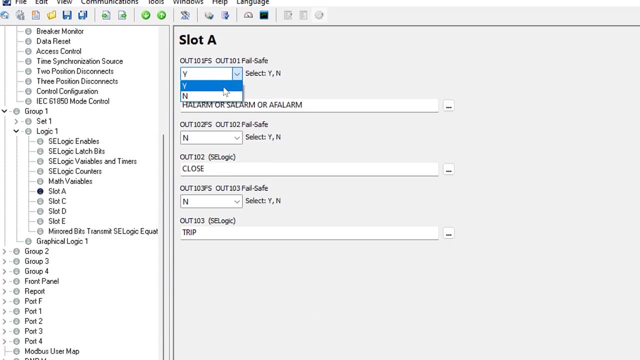 So we're going to have two outputs. we set that output 101, and I can find the outputs over here under group 1,, logic 1, and slot A. I'm going to change this failsafe to a no and for this example, output 101 is going to be our breaker failure lockout trip. 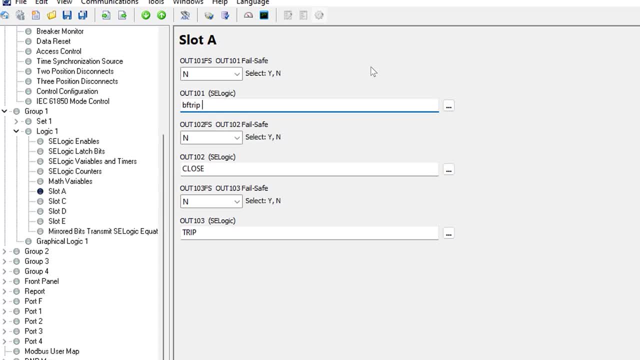 So I'm going to program this to bftrip, which again was the output of the built-in breaker failure trip equation, the one that's sealed in until you manually go and reset it. So this is going to be, and you can put a pound sign for adding a comment. so I'm going. 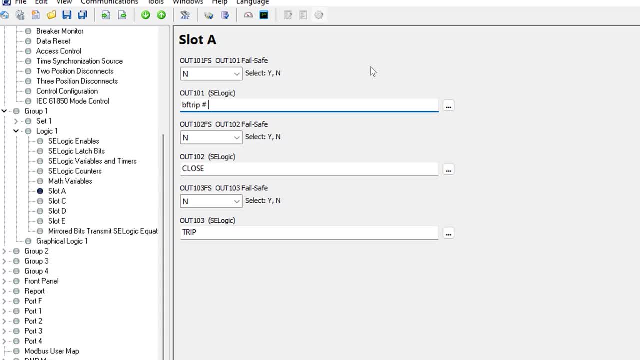 to say bftrip, which is the relay orbit pound, and this is going to be trip bftrip Lockout. So output 101 is going to trip a lockout that is then going to trip all the other breakers, in this case the other four feeder breakers and the two main breakers on the low side. 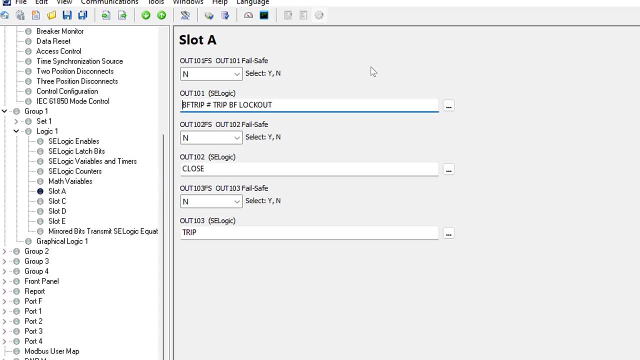 of the transformers. that lockout is going to trip all the other breakers once we declare a breaker failure, trip condition for this feeder. And then, lastly, we set output 102, that's going to be the retrip, that's going to go. 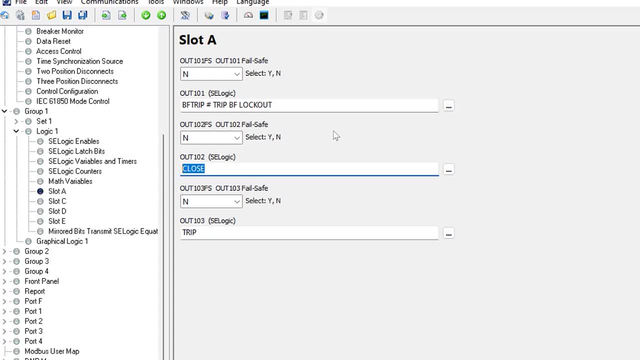 directly to this one breaker. So we're going to set that to bftrip and again, this was the breaker failure retrip orbit. It's a way to try to go ahead and retrip this one breaker only once we receive a successful BFI or breaker failure initiation. 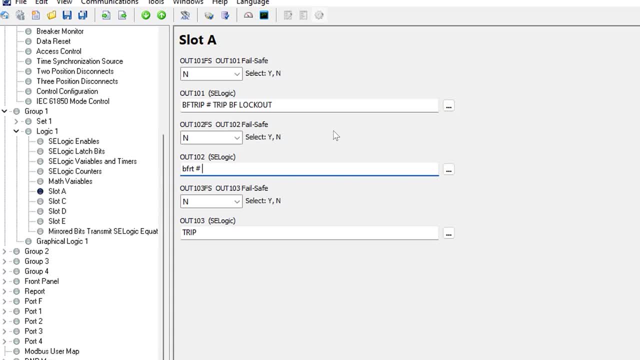 So this is going to be bfrt and I'm going to put a comment here as well. I'm going to say retrip breaker. So out 101 is going to go ahead and trip a lockout which is going to clear the bus once. 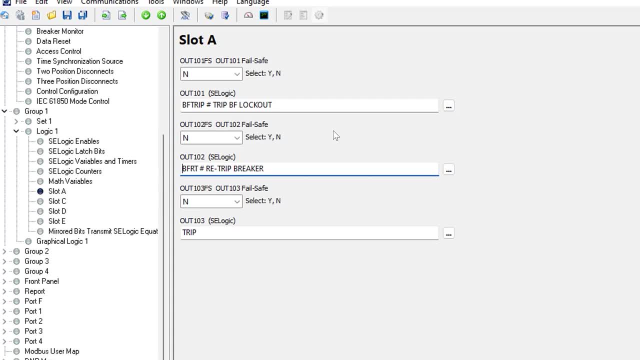 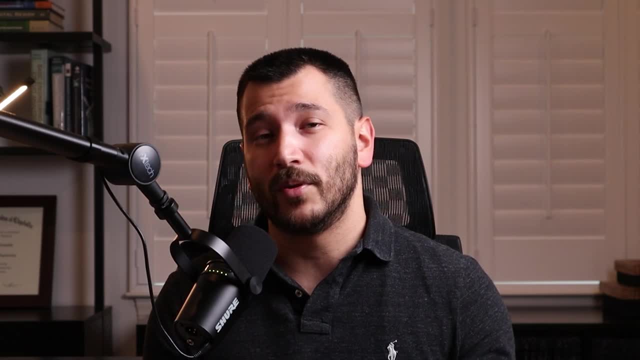 we declare a breaker failure condition and out 102 is just going to trip this one breaker individually. Alright, so that's how breaker failure schemes work. If you want to learn more about logic schemes in protection relays, make sure to check out. 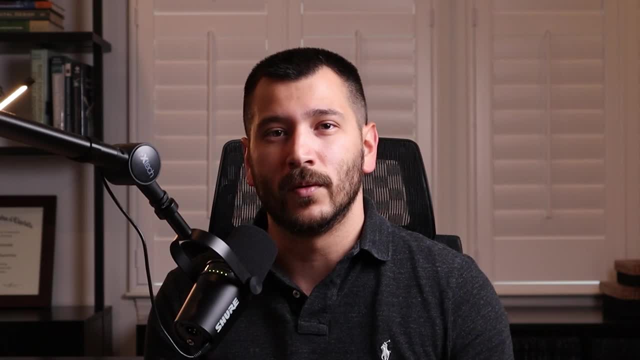 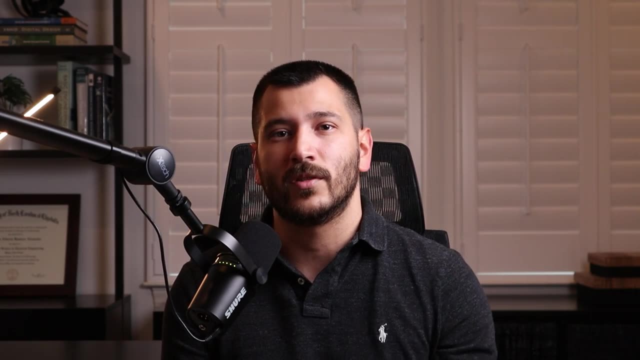 our protective relay logic online course. I'll leave a link in the description below. In that course we go over different logic schemes that we can implement in protection relays, including breaker failure protection and other logic schemes such as automatic reclosing, for example. 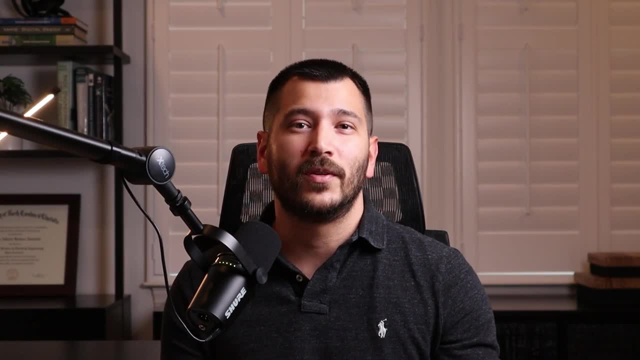 Again, I'll leave a link in the description below if you want to check it out. And, as always, make sure to hit the like button if you found this video helpful and subscribe to the channel for more videos about power engineering and power system protection, and. control, and we'll see you in the next one. 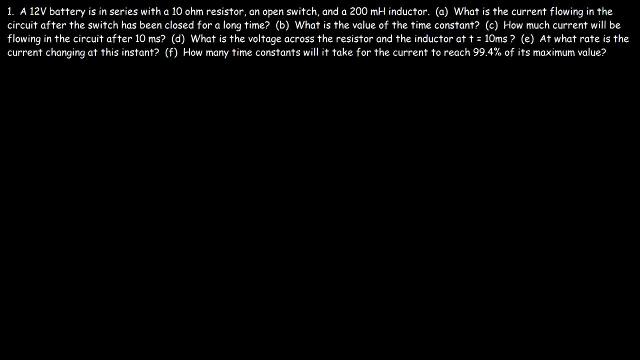 In this video we're going to go over the LR circuit, So let's work on this problem. A 12-volt battery is in series with a 10-ohm resistor, an open switch and a 200 milliHenry.